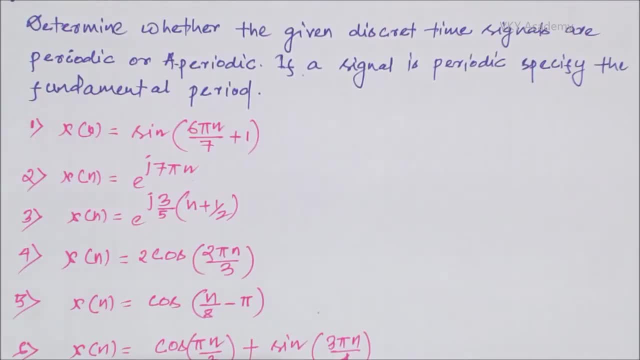 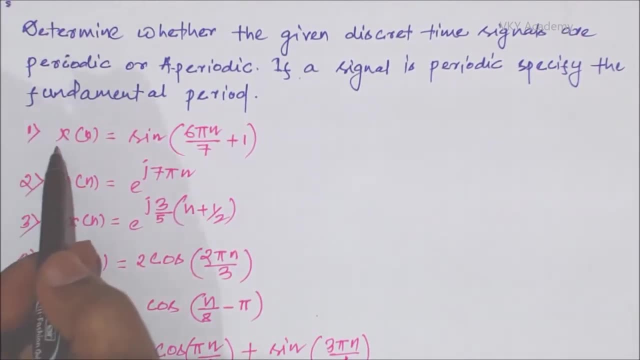 Hello everyone. So in the previous session we have solved a numerical based on periodicity. We solved question number 1, x of n is equal to sine 6, pi, n by 7 plus 1.. And we concluded that this particular signal is periodic with fundamental period 7.. So today we will solve: 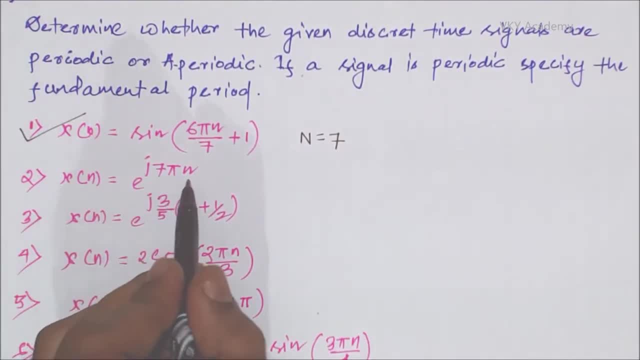 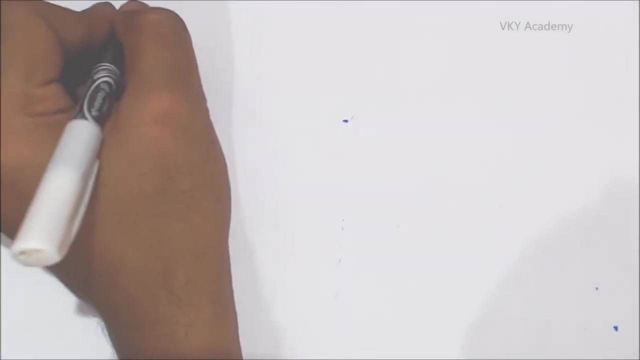 question number 2.. x of n is equal to e to the power j 7 pi n is periodic or non-periodic? If it is periodic, then what is the fundamental period? So let us get started. So my signal is: x of n is equal to e to the power j 7 pi n. So this is an example of complex exponential. 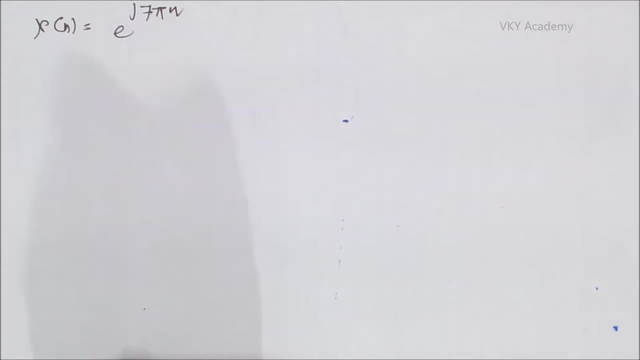 function. Let us check whether this particular signal is periodic or not. Let us assume the signal is periodic with period capital N. If it is periodic with period capital N, then I can say x of n is equal to x of n plus capital N, e to the power j, 7 pi n plus. 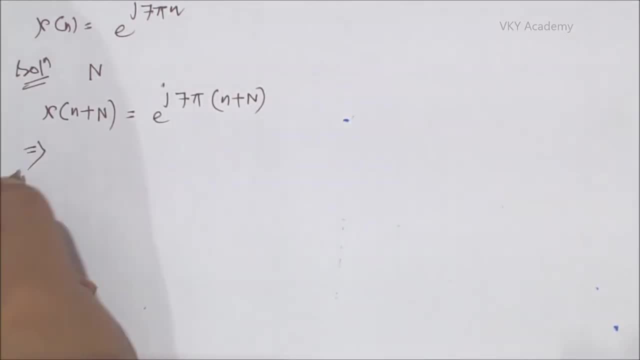 capital N. Now this can be written as: x of n plus capital N is equal to e to the power: j, 7 pi small n plus 7 pi capital N. Now, as we discussed in the previous class, we need to choose the term which contains: 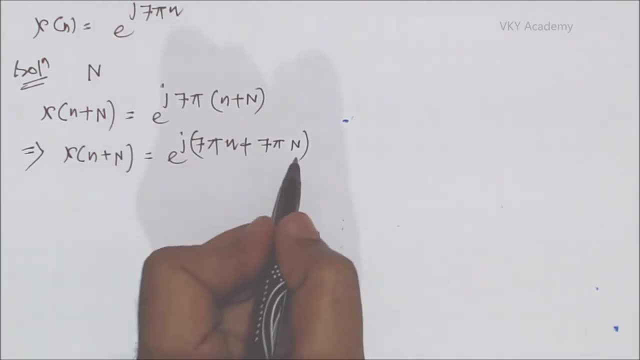 capital N. So in this particular function, this particular term contains capital N, Because we need to calculate, we need to determine the fundamental period and capital N is my fundamental period. So 7 pi capital N is actually omega 0 n, which is 2 pi small m. 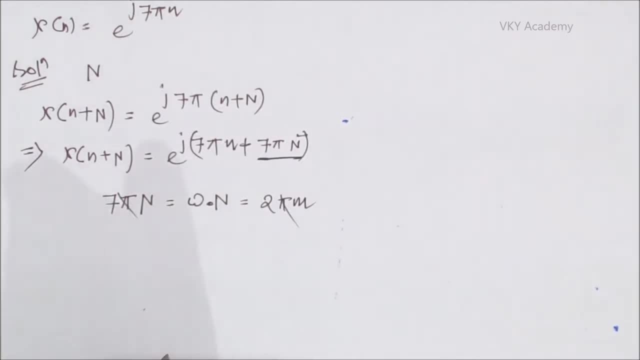 Now pi capital N is equal to x of n plus 1.. So this is an example of complex exponential. now phi and phi get cancelled out. now we have capital n is equal to 2 into small m divided by 7. now what is my next task? my next task is i need to choose the smallest value or smallest integer. 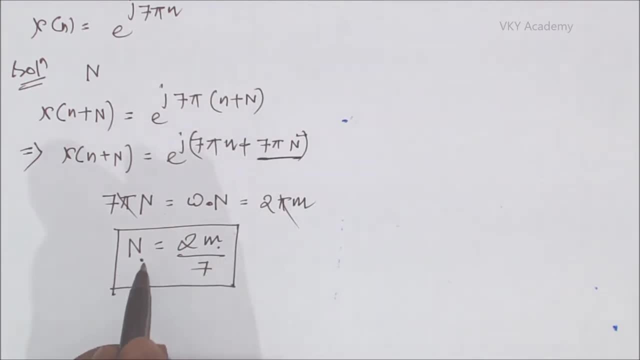 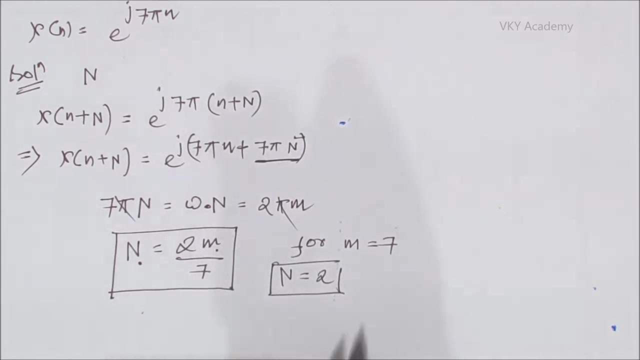 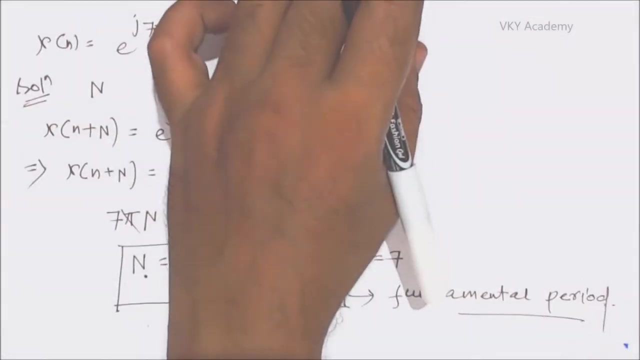 value of small n in such a way that capital n is a whole number, or we can say it is an integer. so for small n is equal to 7, capital n is always equal to 2, so i can say: this is my fundamental period. okay, so in this way we can calculate the fundamental period for a given discrete time. 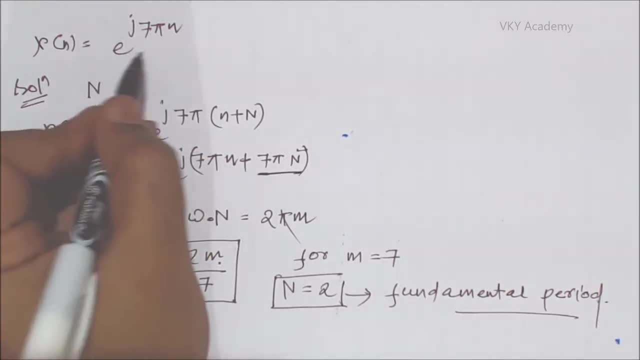 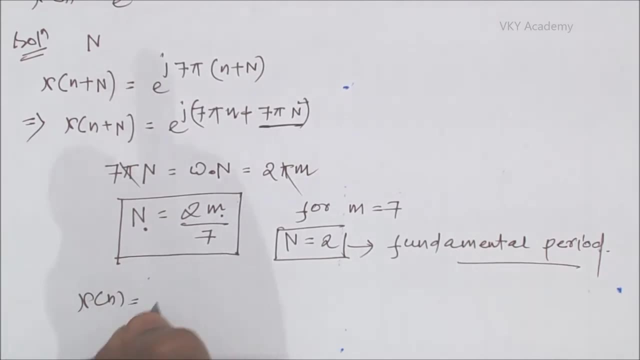 signal. so we have seen here is that we have seen here is that we have seen here is that any exponential function of such type are always periodic in nature. like, if you take an example, x of n is equal to e, to the power minus j, 3, pi, n. 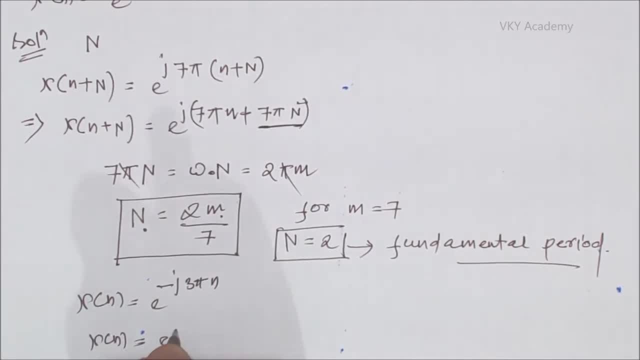 x of n is equal to e to the power plus j, 3 by 2 pi n. x of n is equal to e to the power minus j, 3 by 2 pi n. so these all signals are periodic in nature. so these all signals are periodic in nature. 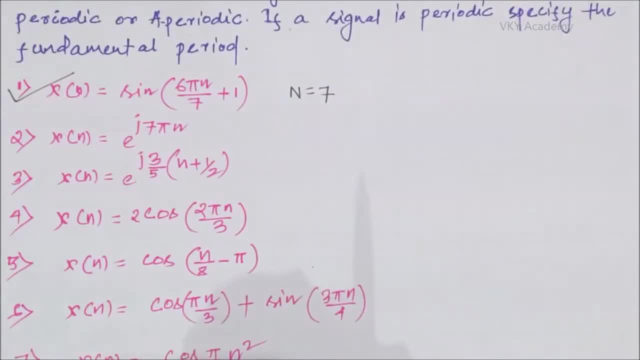 so these all signals are periodic in nature with some fundamental period, with some fundamental period, with some fundamental period. so this particular signal is periodic with. so this particular signal is periodic with. so this particular signal is periodic with period capital n is equal to 2 period capital n is equal to 2. 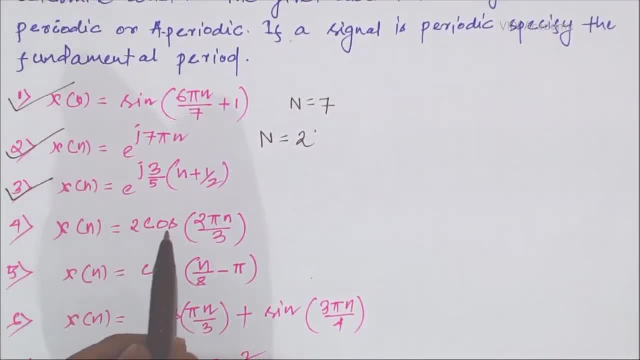 period, capital n is equal to 2. let us solve one more numerical question. let us solve one more numerical question. let us solve one more numerical question, number three. this is also an example of number three. this is also an example of number three. this is also an example of exponential function. let us check whether. 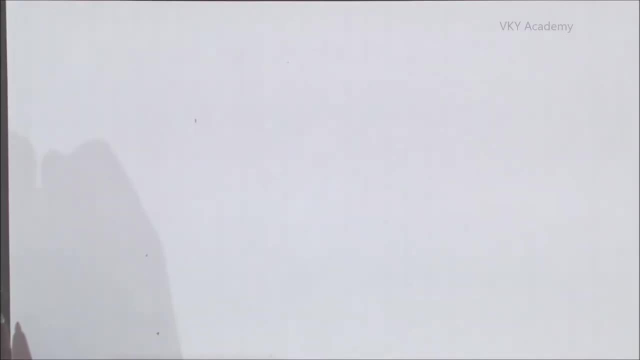 exponential function. let us check whether exponential function. let us check whether this particular signal is periodic, or this particular signal is periodic, or this particular signal is periodic or not, not. not. so my signal is: x of n is equal to. so my signal is x of n is equal to. 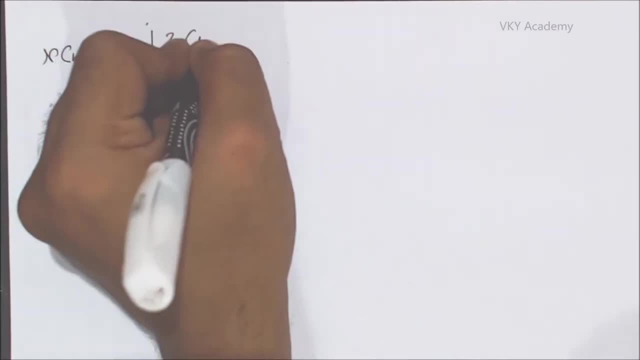 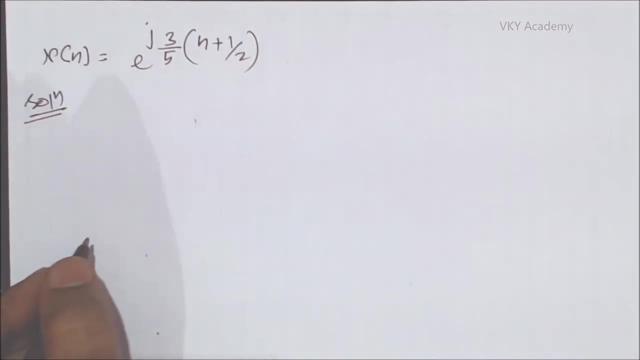 e to the power j 3 by 5 n plus 1 by 2.. Let us assume this particular signal is periodic with period capital N. So I can write: x of n is equal to x of n plus capital N, and that is e to the power j 3 by 5 n plus capital N plus 1 by 2.. That can be written as x of 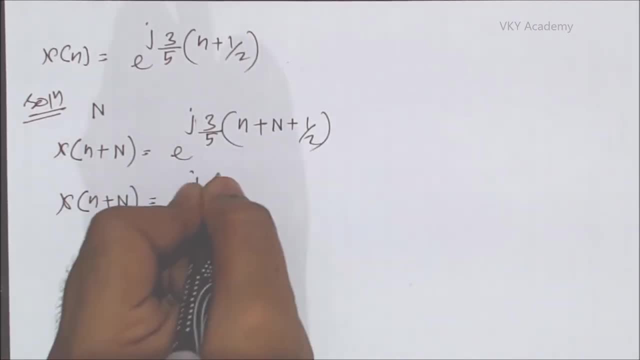 n plus capital N is equal to e to the power j: 3 n by 5 plus 3, capital N by 5 plus 3 divided by 10.. Now we need to focus the particular term which contains capital N, because capital N is my fundamental period. So 3 n by 5 is the term which contains capital N and according 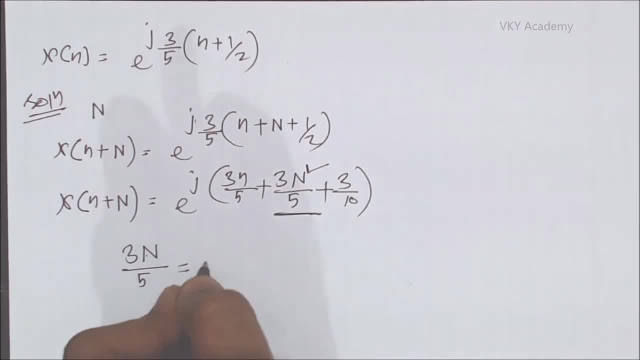 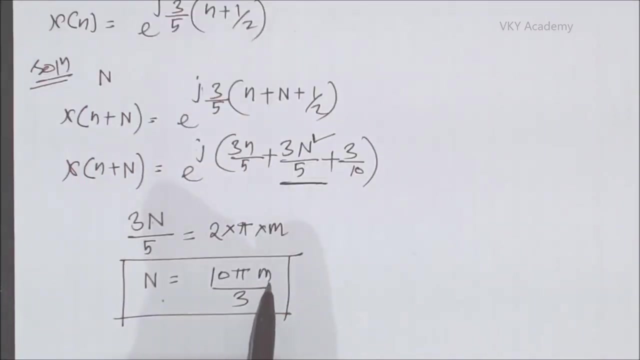 to the condition I can write: 3 n by 5 is equal to 2 into pi, into small m. and finally, capital N is equal to 10 pi small m divided by 3.. Now we need to put a non-zero integer value for small. 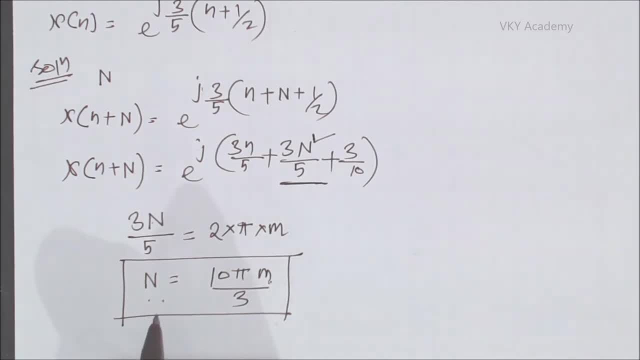 m in such a way that capital N is always a whole number. or we can say capital N is an integer. So for any integer value of small m, capital n is never being a whole number, Just because pi is an irrational number. So we can conclude that this particular signal 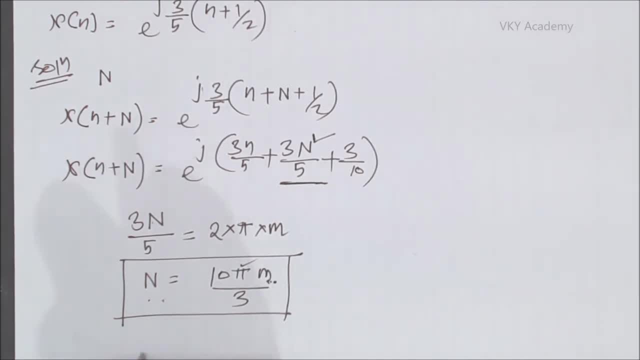 x of n is equal to e to the power j, 3 by 5, n plus 1 by 2 is a periodic in nature. So by solving this particular numerical we got one concept, and the concept is that if pi is not associated with small m as a multiplication factor, then such type of a 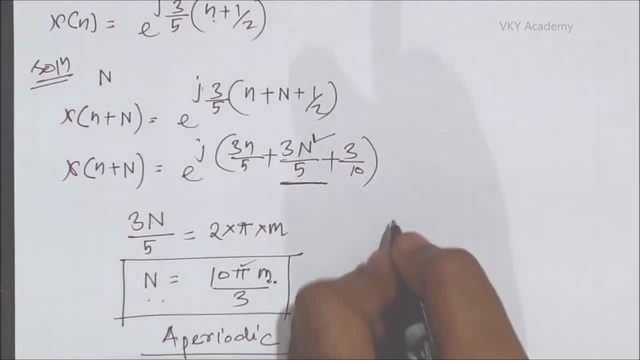 signal are always a periodic in nature. Let us take one more example. x of n is equal to cos 2 pi plus m. This particular signal is also a periodic in nature. Why? Because pi is not associated with small m as a multiplication factor. So if you see any of the signals, 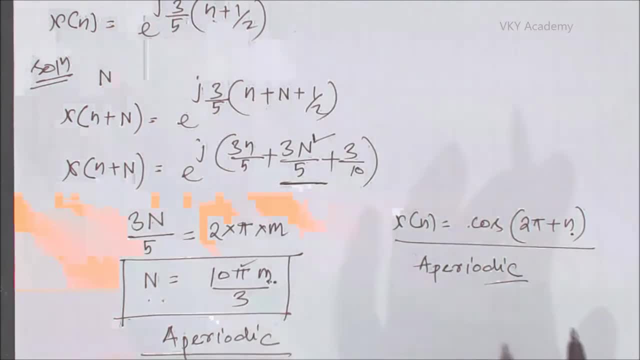 it may be a cosine function, may be a complex exponential function or any type of signal. if you do not see a pi as a multiplication factor with small n, then without any hesitation we can write that particular signal is a periodic in nature. Now, if a signal is of such type, x of n is equal to cos of 2 pi n plus 1.